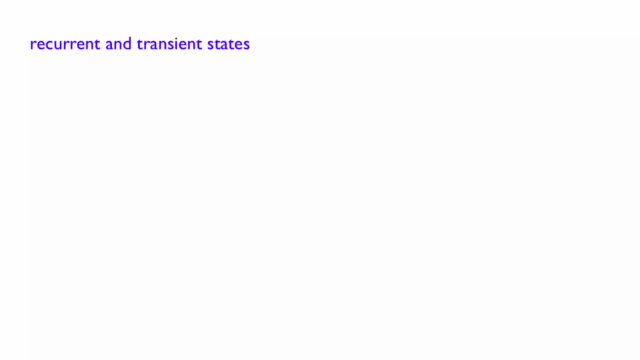 into two types: recurrent and transient. A state is said to be recurrent if, starting from that state, no matter where you go, there is always a path to come back. A state is said to be transient if it is not recurrent. It means that starting from that state, 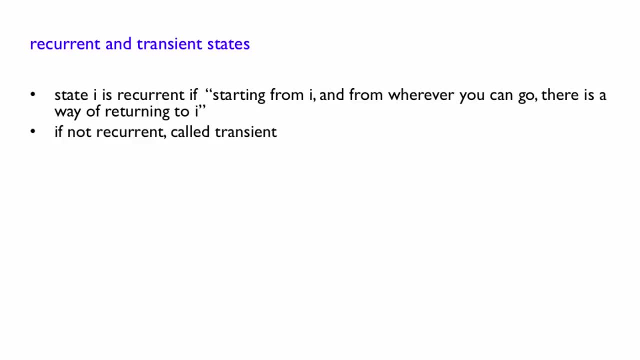 there is at least one place where you can go, and then there will be no path back to it. For example, starting from state eight, no matter where you go, there is always a path back to eight. So eight will be said to be a recurrent state for the same. 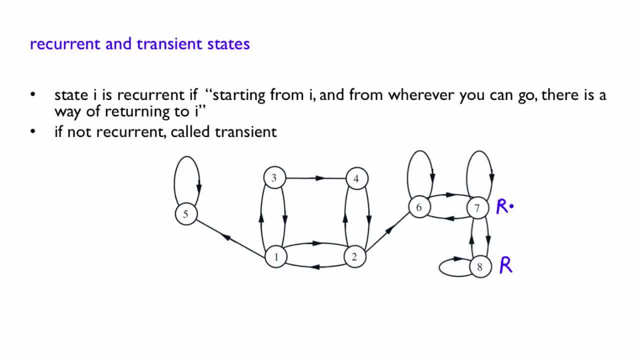 reason. Seven will also be a recurrent state, as well as six. Now what about five From five? the only state where you can go to is five itself, So five is also a recurrent state. Let us look now at a state like state four. 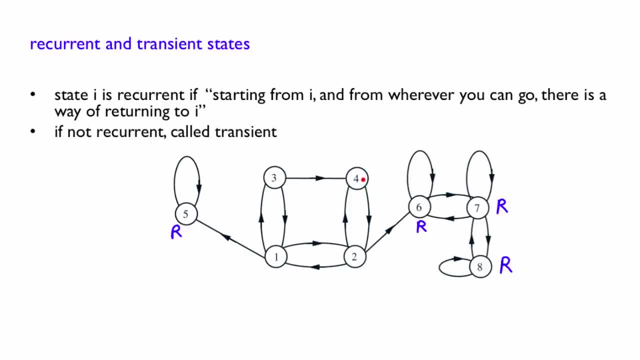 From four. there is the possibility of a path going through two, then one and then going to five, from which there is no path back to four. So four cannot be a recurrent state. It is then called a transient state For the same reason, starting from three. 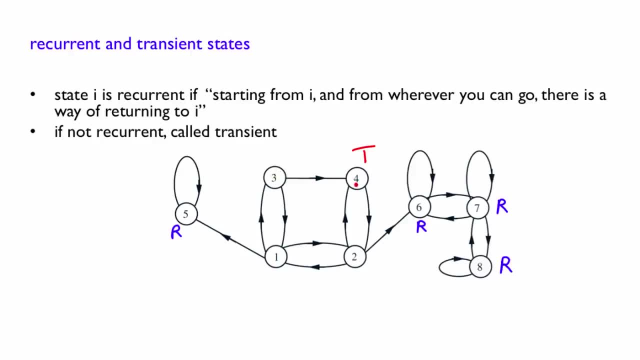 there is the possibility that, after doing many transitions, you will be in either two and then go to six, or you will eventually be in one and then go to five, And from five or from six there will be no path back to three. 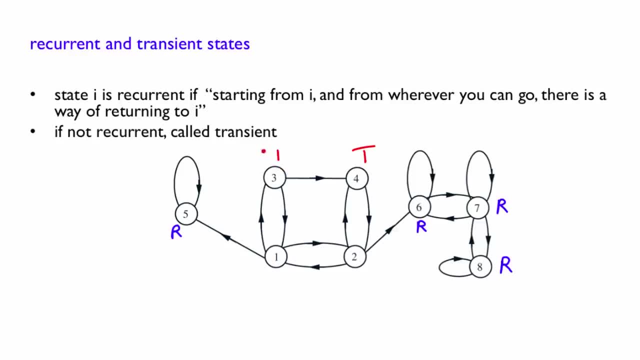 So three is also a transient state And it is clear that, for the same reason, one will be in either two. OK, One will be a transient state and two will also be a transient state. Now, if a state is transient, like three, four or one,